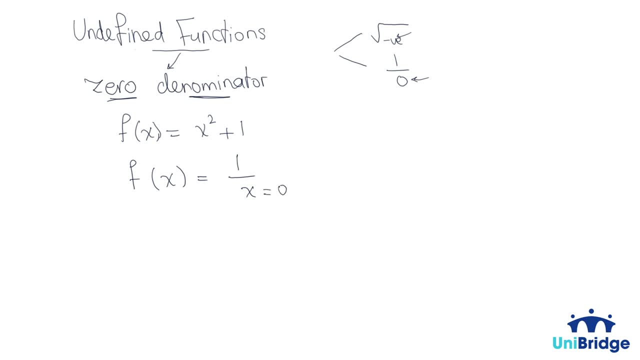 would make the denominator 0,, in this case when x is just equal to 0.. So the way you solve this problem is that you take the denominator, regardless what it is, and you equate it to 0.. Okay, So if you have f of x is equal to 1 over x minus 3, and the question is stating: 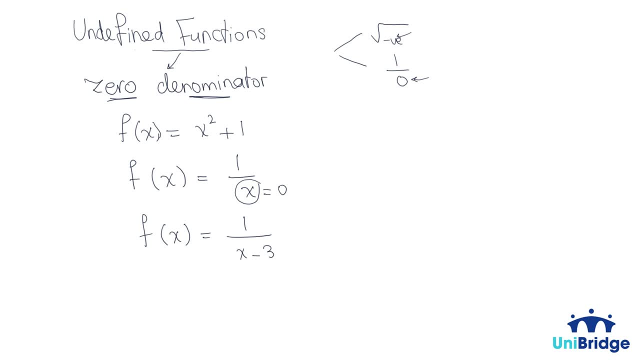 for what value of x will this function be undefined? So if you want this function to be undefined, so you take the denominator and you equate it to 0, so you do: x minus 3 is equal to 0. And then you solve for x. So what value of x will make this equal to 0 when x is equal? 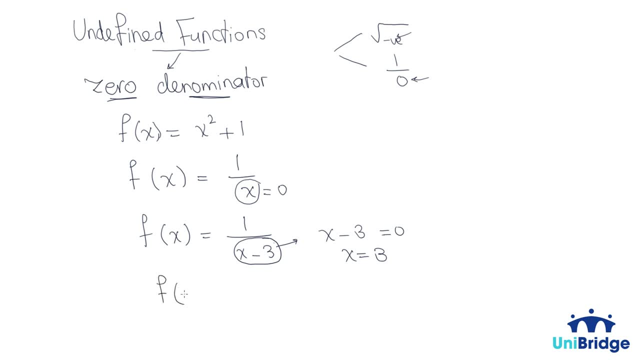 to 3?? Okay, If we take a slightly more complicated question, let's say you have 1 over x, squared minus 4.. And again it's saying: for what value of x will the function be undefined? So again, all we do is we take the denominator and we equate it to 0. And we just solve for x. 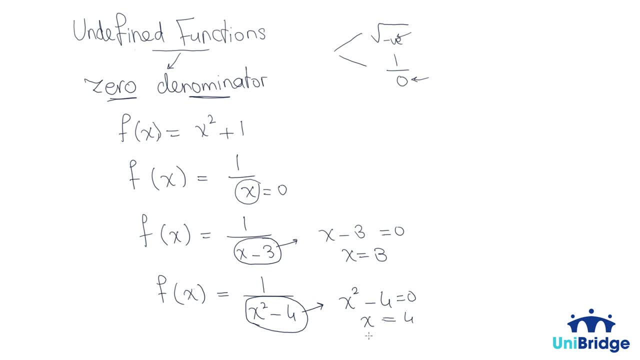 So that will make this denominator equal to 0.. So in this case, this is x squared equal 4. So x is going to be positive or negative, 2. If you have an example that looks a little bit more complicated: if you have something like this, then again, if you want this function, 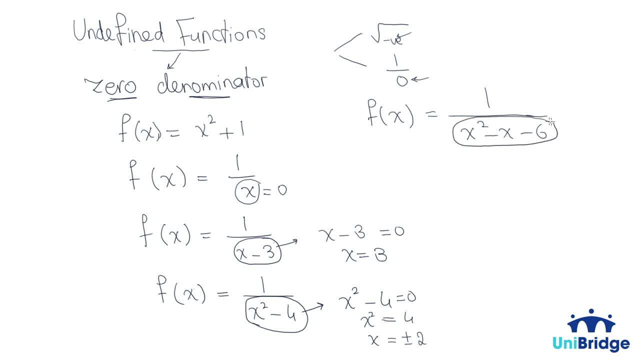 to be undefined. so you're going to take the denominator and you're going to equate it to 0.. Okay, So you get something like this: x squared minus x minus 6 equal to 0. And then you can go ahead and factorize. So this is going to be x and x. We said that we look at this sign. 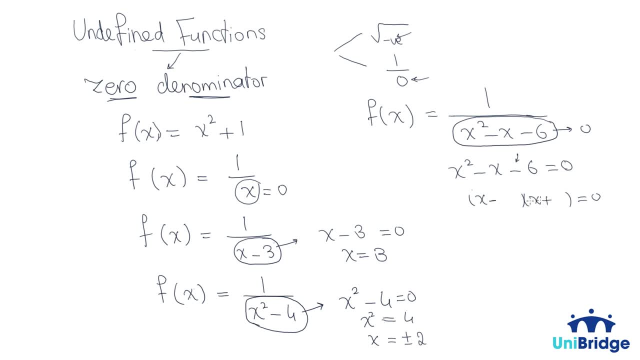 If this is negative, then 1 negative, 1 positive, And the multiplication is going to be 3 and 2.. So you're going to get that either x is equal to 3 or that x is equal to 2.. So you're.